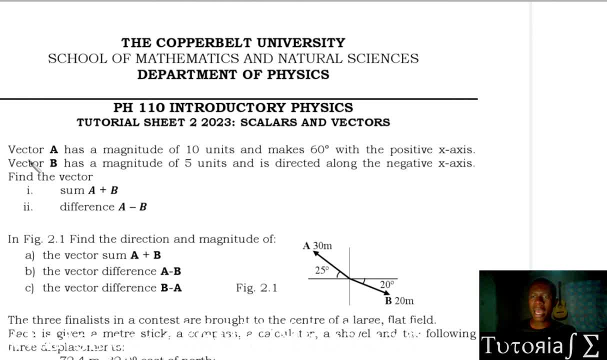 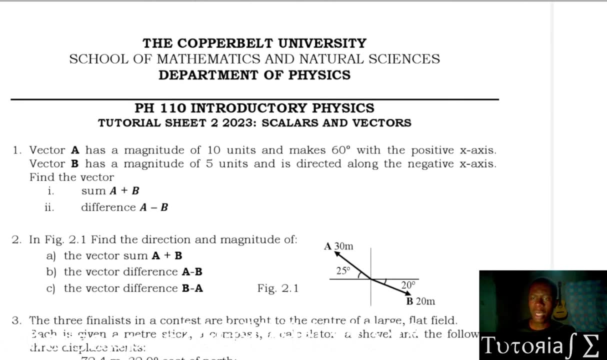 Alright. so question number one here reads: a vector a has a magnitude of ten units and makes 60 degrees with positive x axis. alright, Just move it a bit here. Vector a has a magnitude of ten units and makes 60 degrees with positive x axis. then we have vector b that has a magnitude of five units and makes six degrees with positive x axis. So the으니까 is bequeathed, theka is bequeathed. So it will provide that to you and it will give you verification on the greatest exercising. 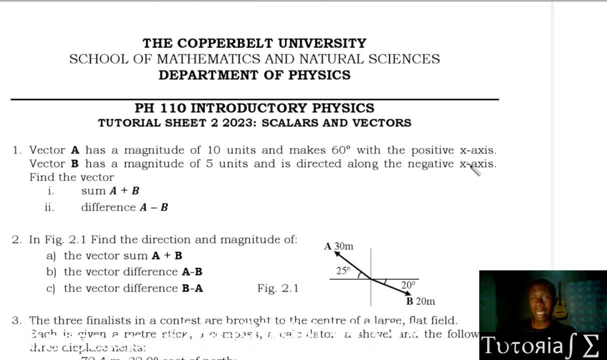 method possible makes and is directed along the negative x-axis. So, basically, what we have here is a simple question and, for physics, what you want to do is you want to first try to transcribe a diagram from the question, or transcribe the question into a diagram. That way, it will be easier for you to solve the. 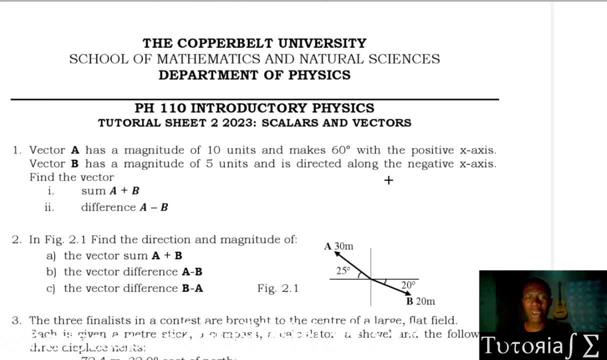 question. So, me transcribing this question into a diagram, I would have to draw an x or y plane. Let me draw it in red. Let me draw my x or y plane in red. So I would have to draw an x or y plane. 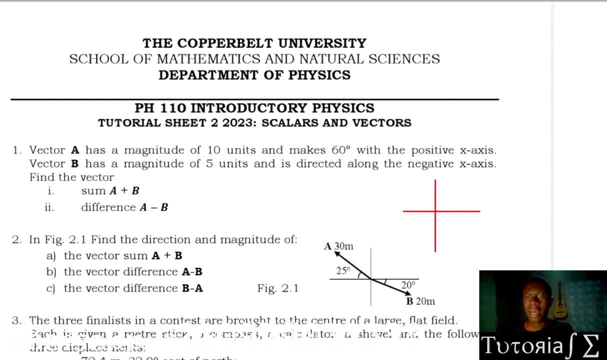 like that. Then a is 60 degrees, So this segment on the x or y plane are in 90 degrees. So this is a x or y plane. So I would have to draw a x or y plane in red. So I would have to draw a x or y. 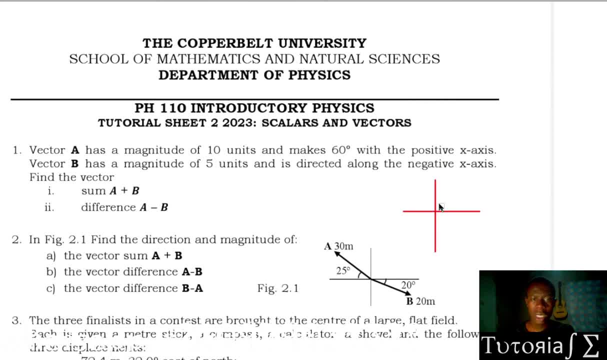 90 degrees. I mean this is 90 degrees, This is 90 degrees, This is 90 degrees And that is 90 degrees And all together that adds up to 360.. All right, So a is 60 degrees, It is 10 units. 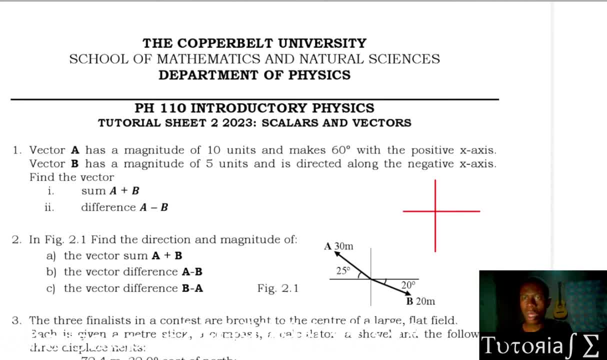 Let me use black for that, All right. So a is that is the magnitude, that is a, that is a and has a magnitude of 10. And is that 60 degrees from the x axis. then we have b, that is five units and is along the x axis. So that is five units along the x axis. that will be. 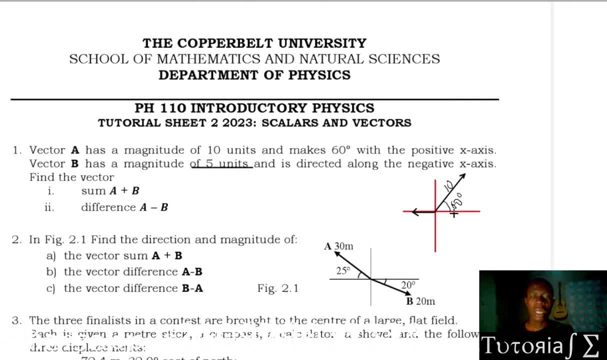 along the x axis. So that is five units along the x axis. So that is five units along the x axis axis, five units like that. so how we count, or how we count angles for vectors, we always start from the positive x axis when determining the angle at which the vector is at. okay, so when determining, 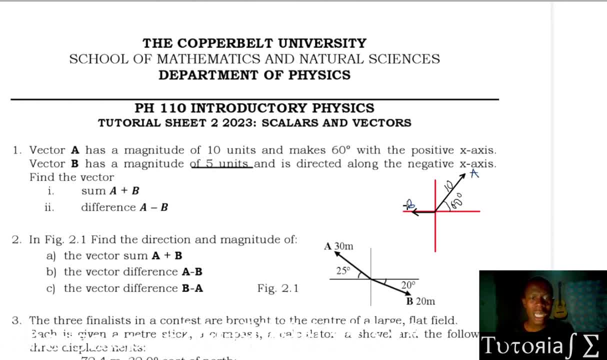 the angle at which the vector is at. we always count from the positive x axis until we meet the vector. so for instance a, we count from this point to where the vector is at. so for b, it will be from this point to where the vector b is at. so that angle, that is 180 degrees there, all right. so 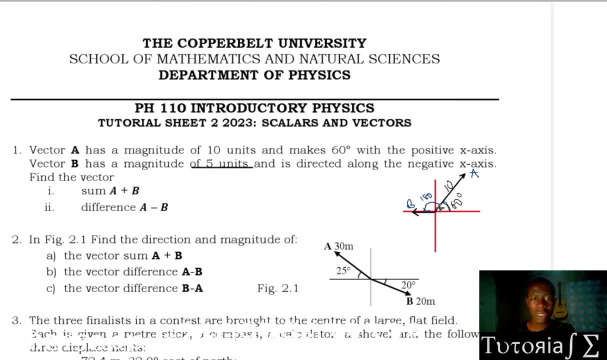 those are the angles. so from here to there, that is 180 degrees. so that is 90 plus 90, 180. from there to there, that is 270. from there to there, that is three. from uh here to there, that is 270. from here to there, that is 360, like that. so these are the angles of a and b. so now for us to add. 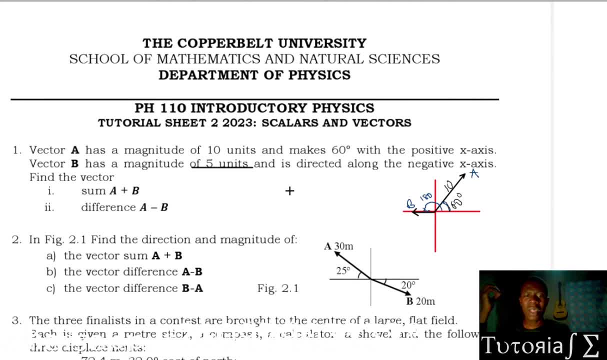 or subtract vectors. we have to reserve the vector a into two components. so: a- for it to be added, it should have an x component and the y component. same applies for b to be added to a: it should have an x component and the y component. now how are we going to do that? so we are going to 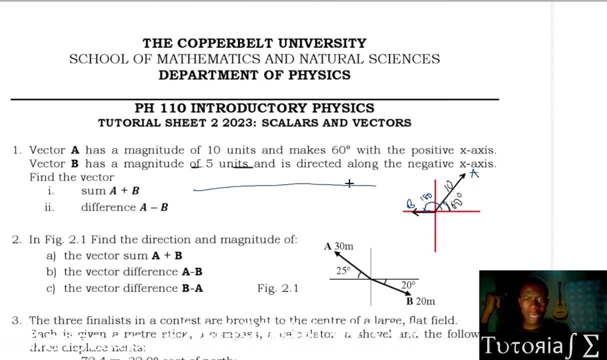 create a simple diagram that i'll just make here. so that will be x, say x, com component, and that is y component, and for each of these components we have our a and our b. there, all right. so for a and for b, we have our x component part and y component part. when we do this, it will help us to. 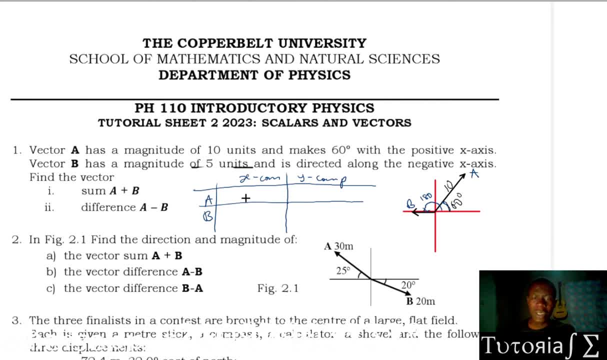 find our x component part and y component part and we will be able to find our x component part and we will be able to find the sum. all right, so for the x component of a, for us to find the x component of a, we look at where a is, so we get the magnitude of a. so the magnitude of a is 10 units. 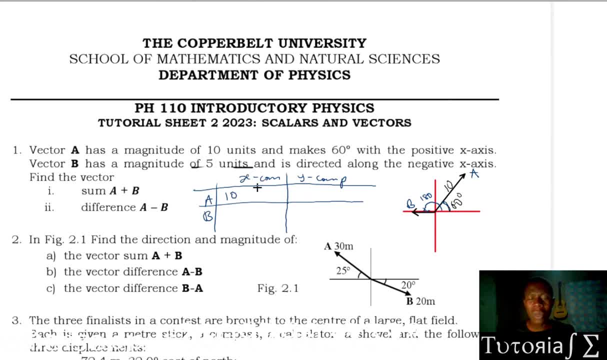 so we write there 10 units. then for x components we always use cos. so we say cos where the a is, or the direction of a. so a is at 60 degrees. remember we always count from the positive x axis to where a is. so from this point to that point, that is, we've already been given that is 60 degrees. 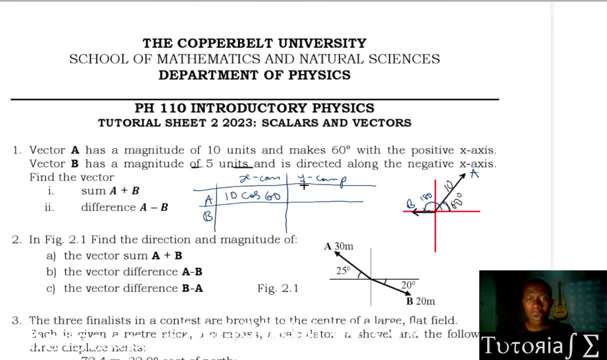 so that is 60 degrees. then to find the y component of a we again write the same magnitude, which is 10. then what changes is just here? so now we are using sine 60 degrees. so that is the x component and the y component of a. so for b we do the same thing. we look at the magnitude of b, so the 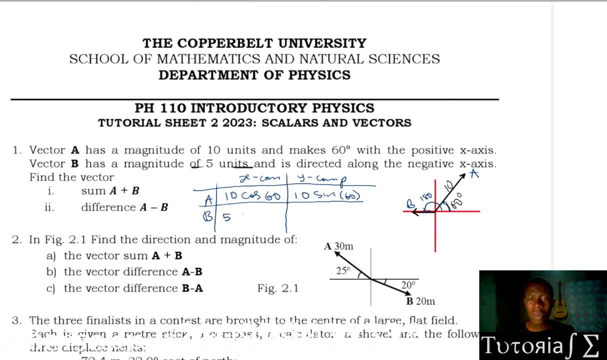 magnitude of b is 5. so for the x component we say cos the angle at which b is at. so we count from positive x axis until we touch b there. so that is 180. so we do the same for the y component. we write everything the same, we just change the cos to sine 180 degrees and that is just about it. so 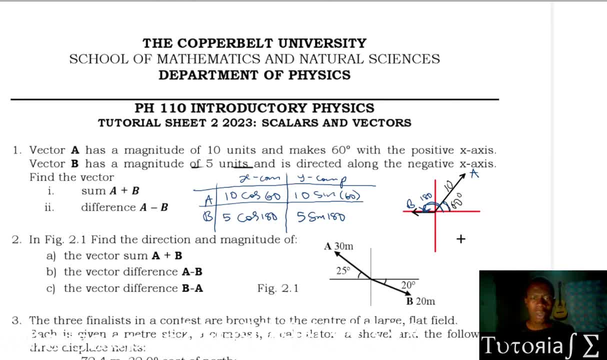 from here. now, what we're going to do is for b, or let me start with a. for a, we have the x component, which is um 10 cos 60. okay, then um the y component, which is 10 sine 60. so always the x component on top the y, the, the y component at the. 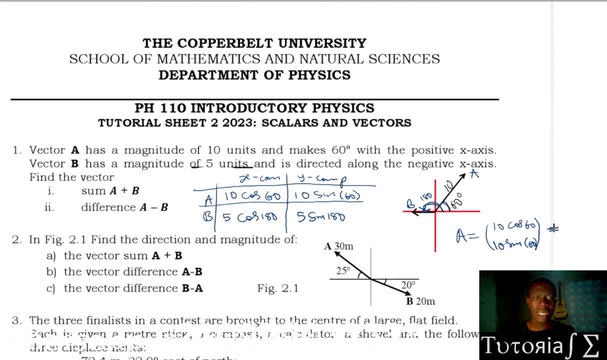 bottom. so now this is actually equal to the x component on top of the y component at the bottom. so when we simplify cos 60, that is half half times 10, that will give us five. uh sine 180, that is 0.8660. so times that, that will be 8.66. all right, so that is a, a. those are. 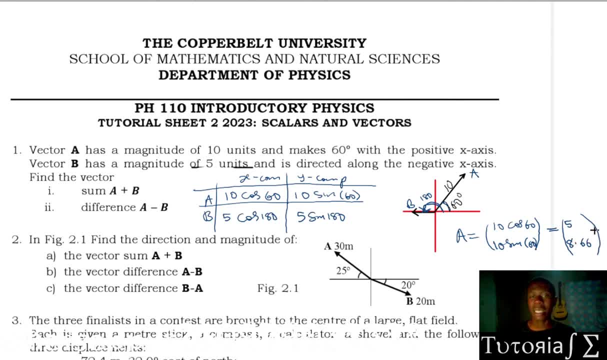 the magnitude, the components five and eight, point six, six. so now we do the same for, for for b. so let me just move this here, i hope you'll be able to see there. so that is a, then for b we do the same, so b will be equal to the x component of b, that is 5 cos 180. then we have 5 sine 180. 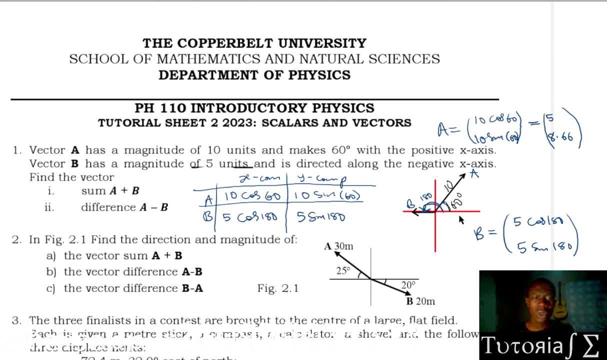 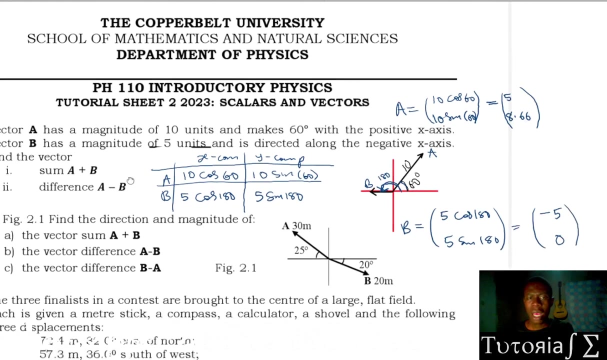 which is, uh, basically just equal to. let me just put it right here: that is just basically equal to five times cos 180. cos 180 is negative one, so negative one times five, that would be negative five. then sine 180 is zero, so that would be zero and um, yeah, so that is basically a and b, then the 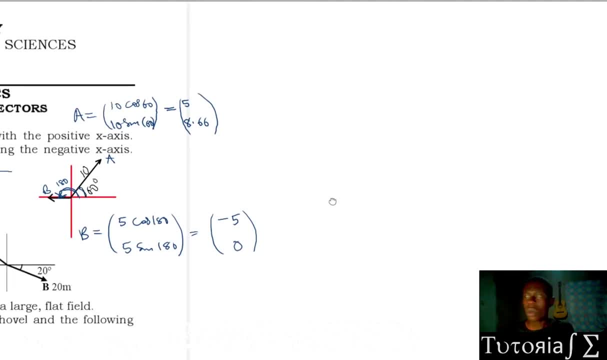 addition part and the subtraction part is very simple, so let me just do it here. so if you are adding, let's say so. let me just put a few examples here. so if you have a plus b, so you start with your a, your a, what is your a here? that is five. 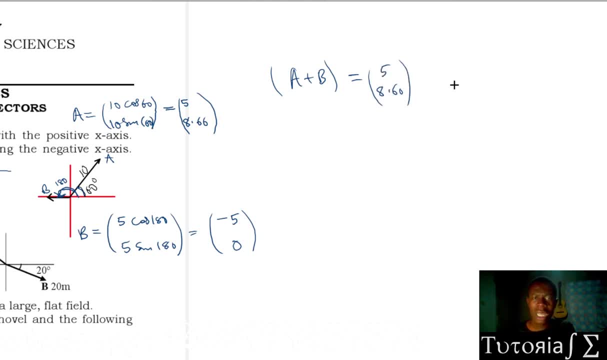 and eight point six six. all right, plus what is your b, that is a negative five and zero there. so adding the two will get this. so we add across. so five plus negative five, that will give us zero. uh, this is six six. eight point six. six plus zero, that will be eight point six six. 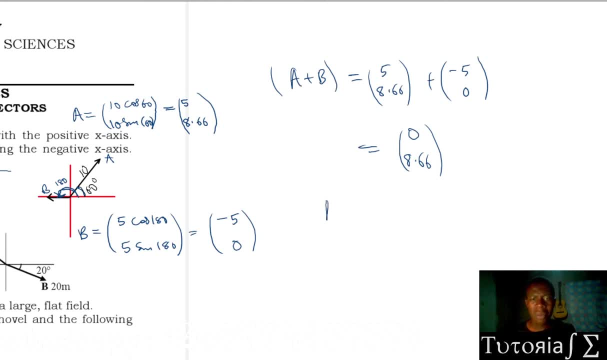 all right, and that is the sum a plus b. for the same reason, when you have a minus b, you start with your a. here your a is a five comma eight point six. six minus your b is negative five and zero. so you do the addition there, so you do the. 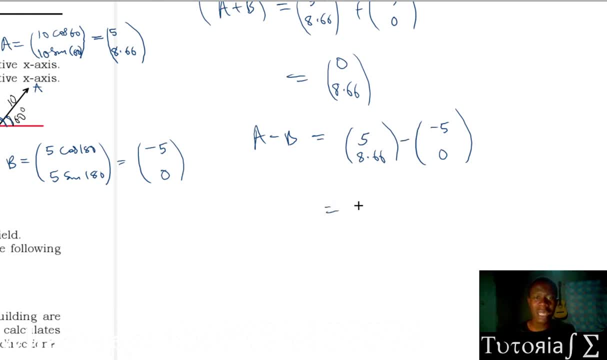 that will be 5 minus minus 5, so that will be 10. then 8.6 minus 0, that will be 8.6. so that is your addition. another example that is not there: maybe you have b minus a. again you do the same thing. 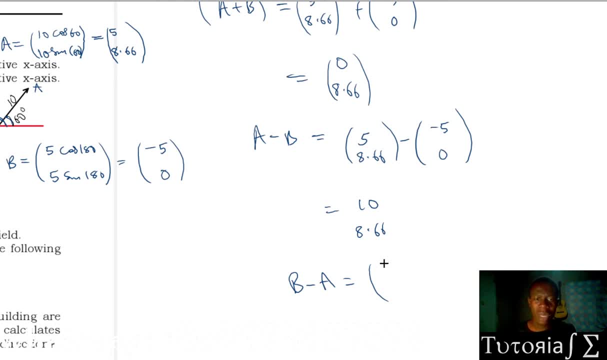 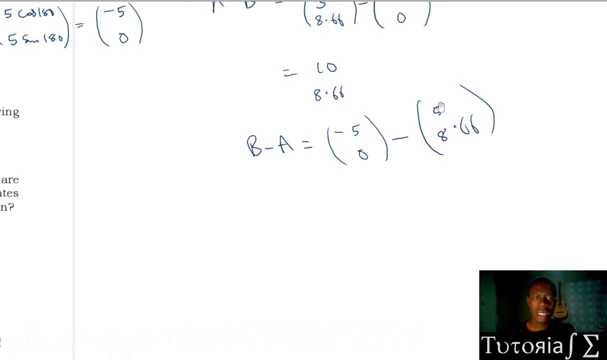 you start with your b. in this case, of this is our b negative 5 and 0 minus our a, which is 5 comma 8.66. let me just put it up there: 866. then you just do the same thing that we've been doing. 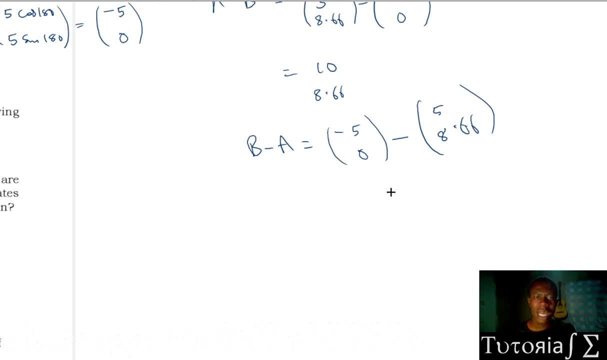 which is, uh, this minus that, that will be negative 10, this minus that, that will be negative 8.66. and that is basically what vector addition. so this is the process that will be taken for adding two vectors or subtracting two vectors. now we come to the issue of finding the angle of the vector or the direction of the vector. 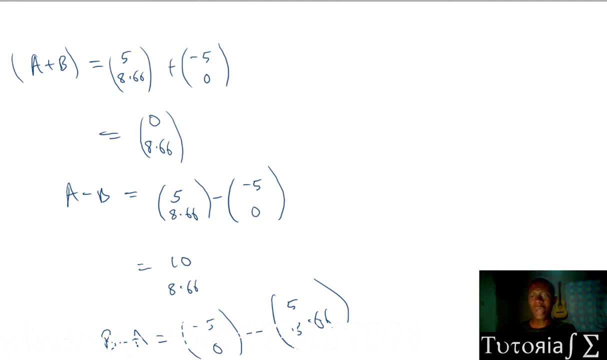 all right, so what for whatever vector that you have, for you to have or for you to find the direction? so, for instance, this vector has a component, the x component, and the y component, that is, a plus b, a plus b has the x component and the y component, and you want to find the 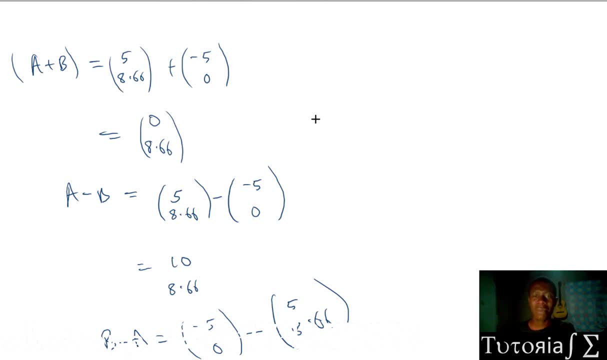 direction of a plus b. so to find the direction of plus b, you have this: a plus b. so the direction is just the angle of a plus b, which is equal to theta, which is equal to the tan inverse of the y over the x. all right, so in this case, 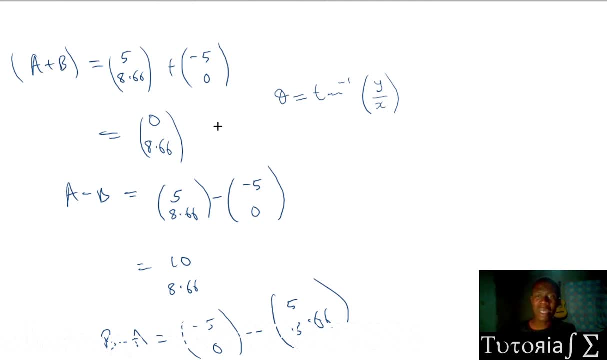 if we're looking at the direction of a plus b, our x is this part, the zero, then our y is this part. so theta will be: goes to the tan inverse of y, which is uh, which is y. what is y here? y is um, y is 8.66 divide by 0, and this is undefined. when you punch this on your calculator, this is: 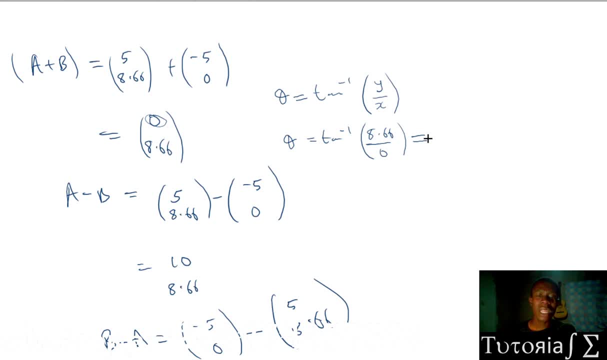 undefined. when it is undefined, we know that the angle at which it is at for tan, that is 90 degrees. all right, so this is at 90 degrees. yeah, so if it is undefined, like in this case, we know that the angle is at 90 degrees. so that will be the direction of 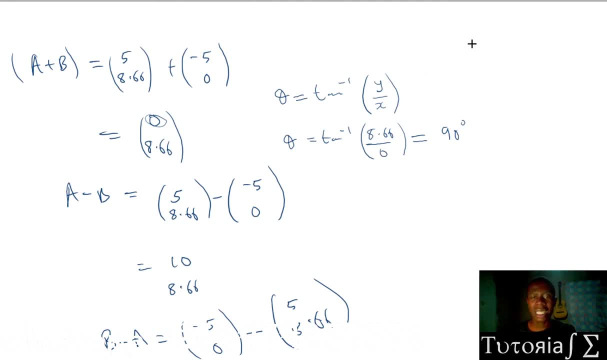 this one. it is at 90 degrees. this is because tan has asymptotes at 90 degrees and 270. so since this is positive, um, so we are in the positive 90 degrees. if we had a negative there, then if we had a negative here, then what would have is a 270 there. all right, so that is. 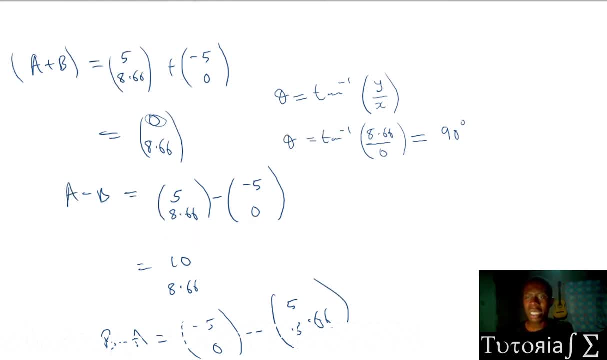 the direction of a plus b. so you do the same for a minus b. a minus b. so that is theta is just equals to the tan inverse of the y axis. let me just show this. why am i missing that? all right, the y axis, which is 8.66. then divide by: 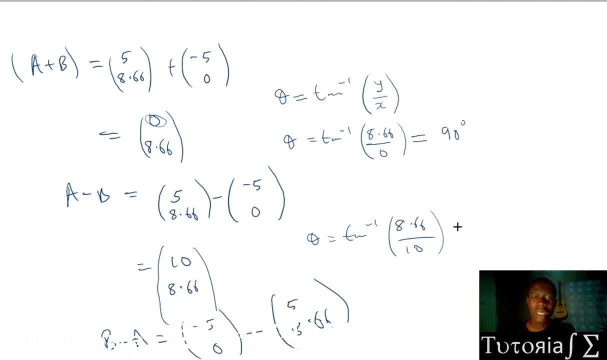 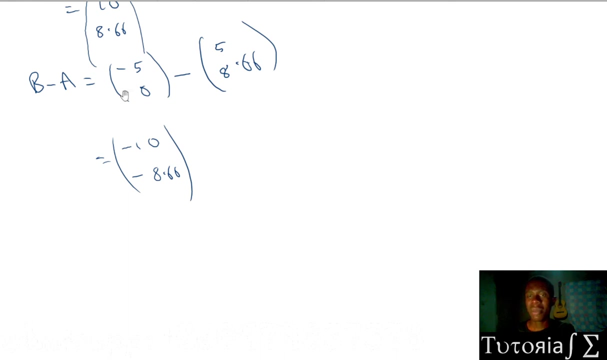 the x axis, which is 10, then you just compute that on your calculator. tan inverse of that, you punch and that will be your answer. so that is how you find the direction. then come into the magnitude. so the magnitude will be this: um, just similar. so for for. 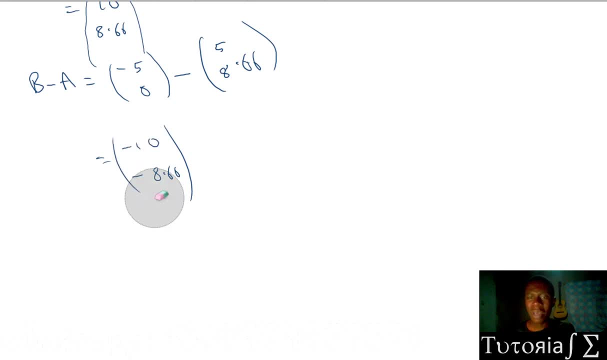 you need to have a vector in this form first of all. so if you have in a vector in this form, then the magnitude, for instance, this is the vector a minus b. i mean b minus a, b minus a. the vector of b minus a is negative 10 and negative 8.66. 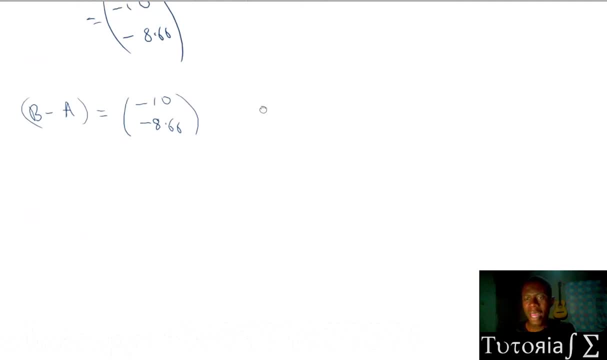 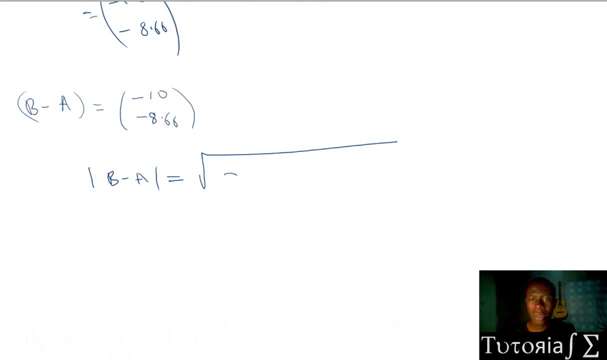 root of the x part, which is this part. or let me just write the formula: the square root of the x part plus the square of the y part, so the square root of the square of the x part plus the square of the y part. so that would be the magnitude. so in this case, x squared, that would be negative 10. 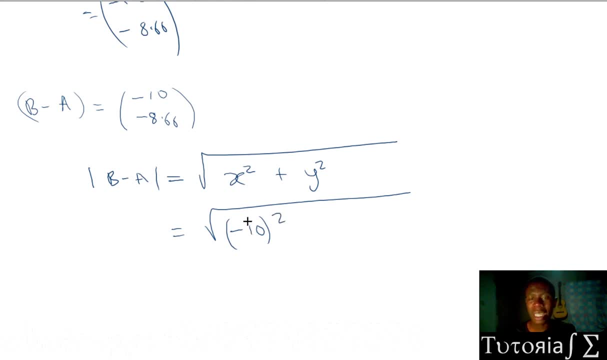 squared. so on your calculator you should be very careful put that in parentheses. so negative 10. then you put the brackets, then you square plus y, which is negative 8.66, then you square as well. so put that in brackets. so negative 10 squared plus that squared, then you find the root of the. 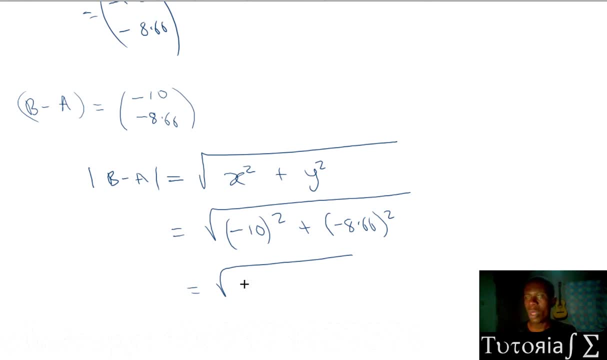 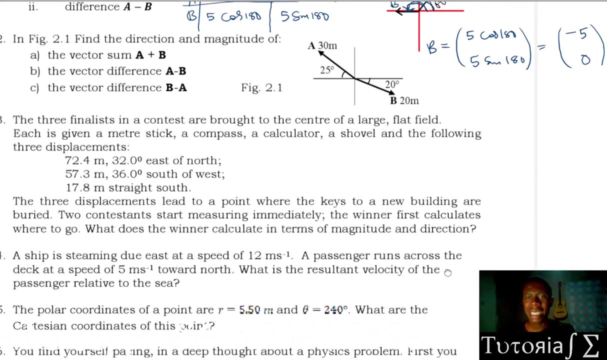 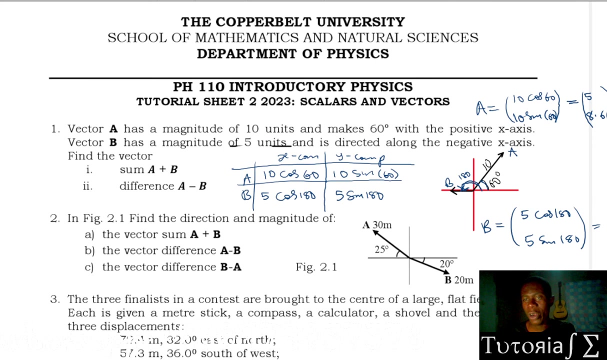 answer and that will be your magnitude. all right, so when you simplify that on your calculator, that will be your magnitude. so this basically explains question uh, question one and two. so question one and two are already so just from the explanation there. so go through the video so to find the direction i've explained. 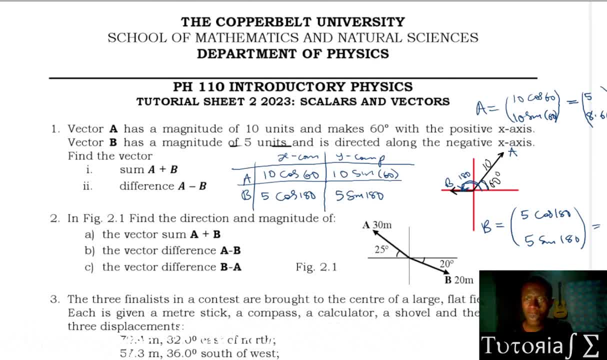 so this is the vector that we have. so for for a, let me just help you. for a, the angle at which a is at is this angle, from the x-axis to where a is. so this entire line is 180 degrees. okay, so if this is 180 degrees, what angle can that be? so that is 25, 180 minus 25. 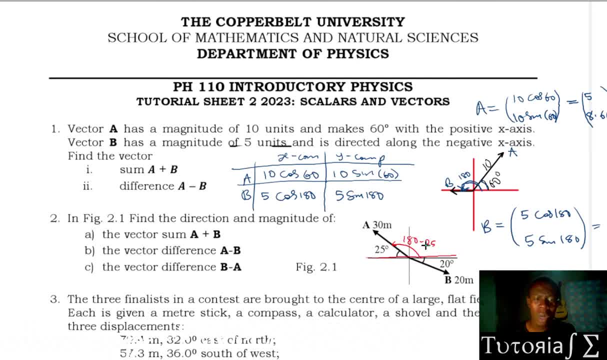 degrees. so this is the angle. this is the angle 180 minus 25. that will give you the angle at which a is at, and for you to find the angle at which b is at, again, you count or you start from the positive x-axis all the way to b. 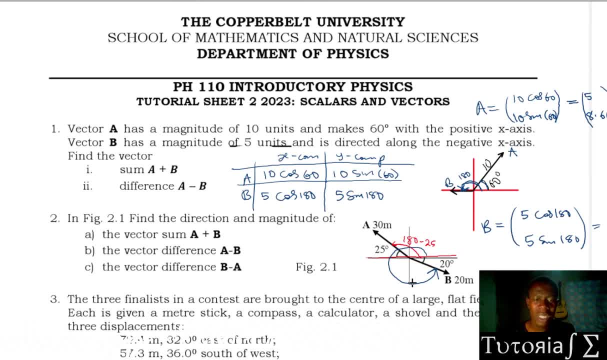 there, all right. so from uh, the positive x-axis, to b, when you reach here, that should give you 360. so this angle is basically 360 minus 20 degrees and that will be your angle for b and you just resolve as we were doing here. so for a you resolve uh, for air, for air you have um 30. 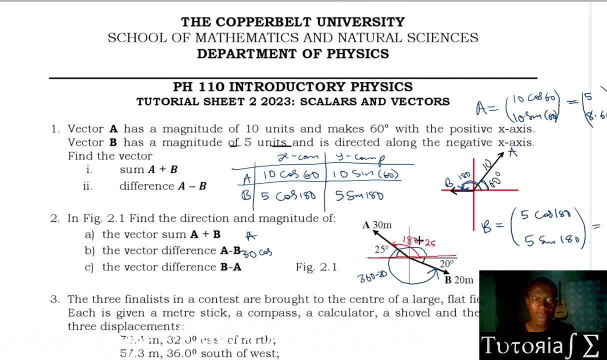 cos um, because what is 180 minus 25? that will be 155. all right, so that will be 155. that is x component, then a y component, that will be. you just get the same thing. so that is 30 cos uh, 150. i mean sine 155.